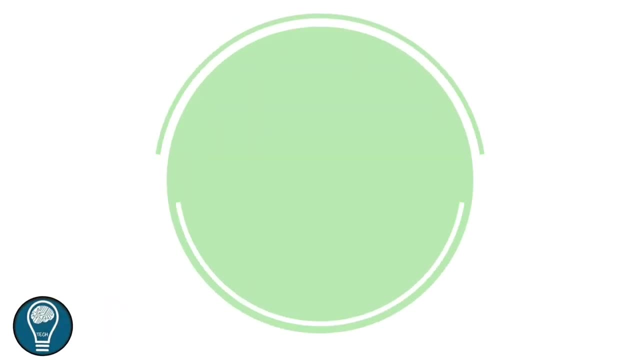 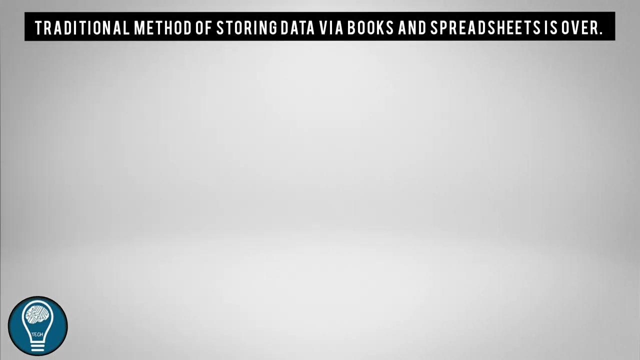 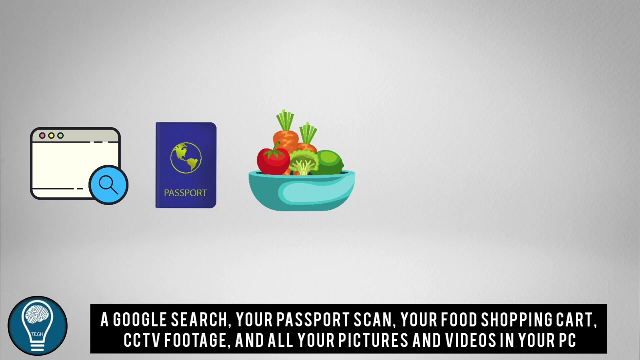 What is Big Data? Table of Content. What is Data? What is Big Data? Characteristic of Big Data and Benefits of Big Data Processing. Traditional method of storing data via books and spreadsheets is over A Google search your passport scan, your food shopping cart CCTV footage and all your pictures and videos in your PC. 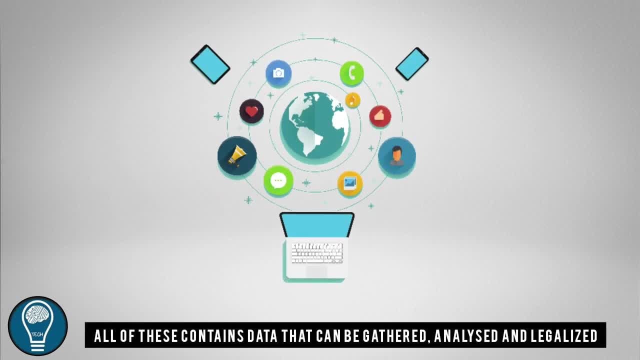 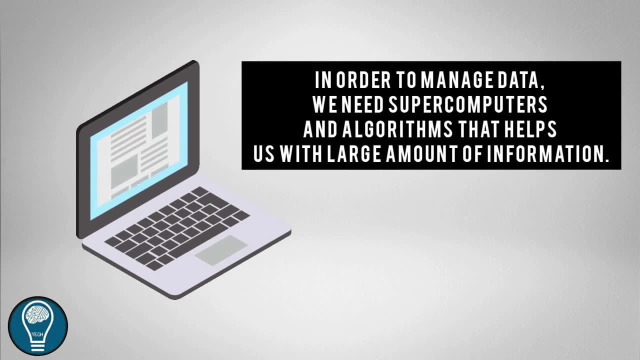 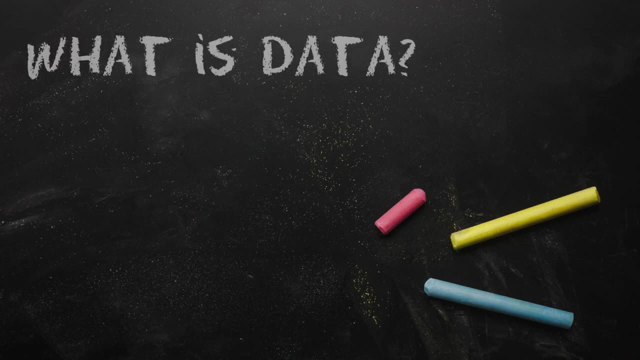 All of these contains data that can be gathered, analyzed and legalized. In order to manage data, we need supercomputers and algorithms. that helps us with large amount of information. In order to understand what is Big Data, we first need to understand what is data. 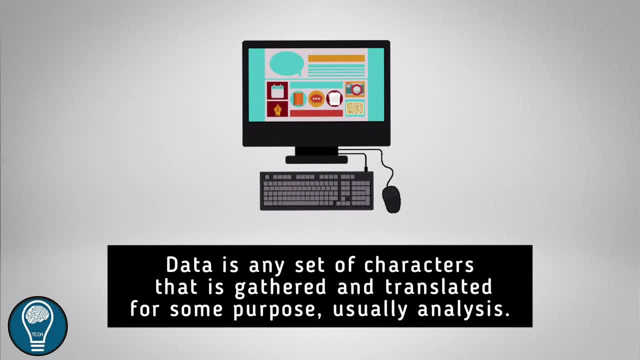 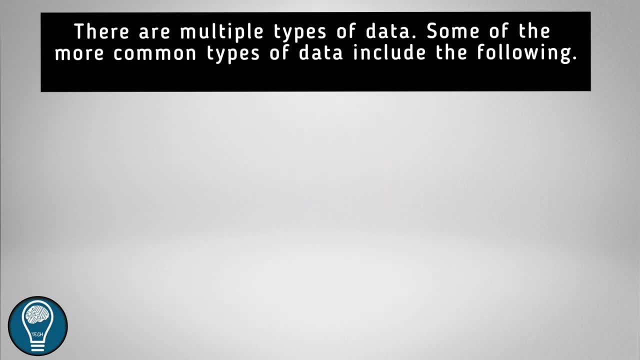 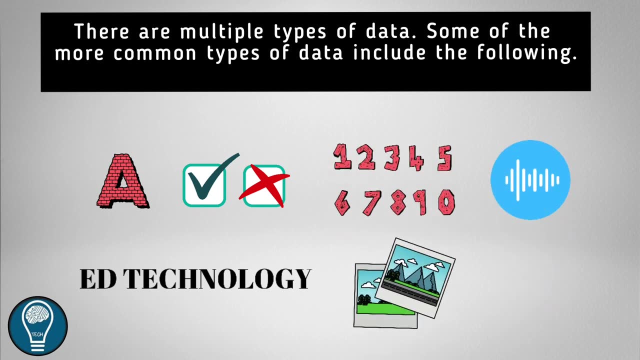 Data is any set of characters that is gathered and translated for some purpose, usually analysis. There are multiple types of data. Some of the more common types of data include the following: single character Boolean text, number, picture, sound, video. 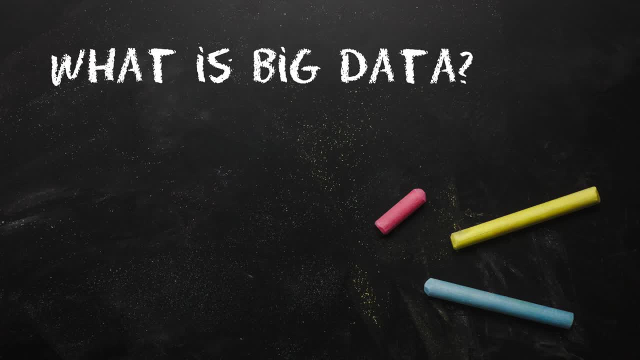 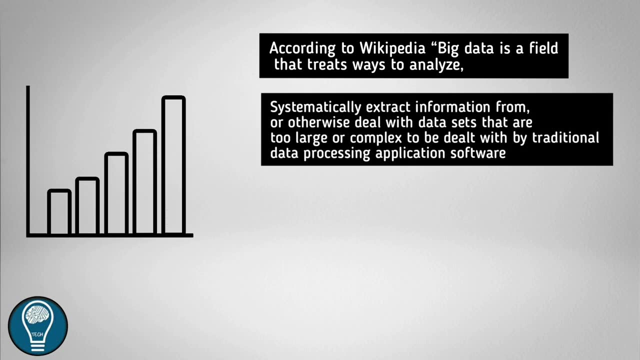 So now let us understand what is Big Data? According to Wikipedia, Big Data is a field that treats ways to analyze, systematically extract information from or otherwise deal with data sets that are too large or complex to be dealt with by traditional data processing application software. 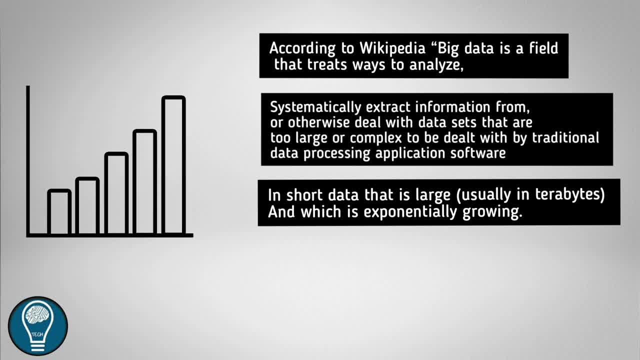 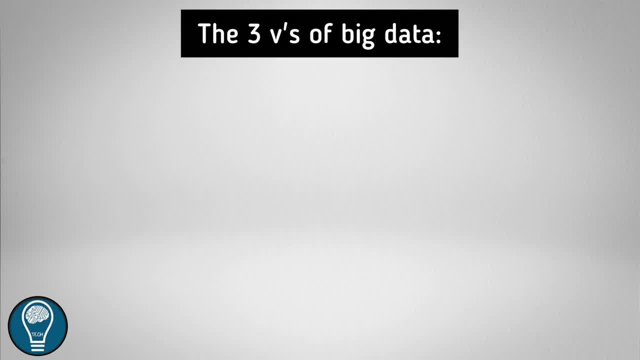 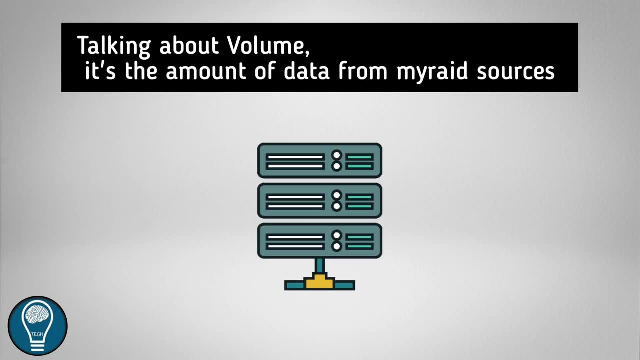 In short, data that is large, usually in terabytes, and which is exponentially growing. Now let us understand characteristic of Big Data. The three Vs of Big Data are volume, variety and velocity. Talking about volume, it's the amount of data from mirrored sources. 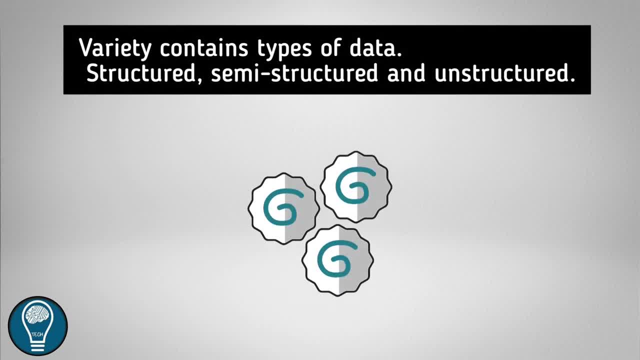 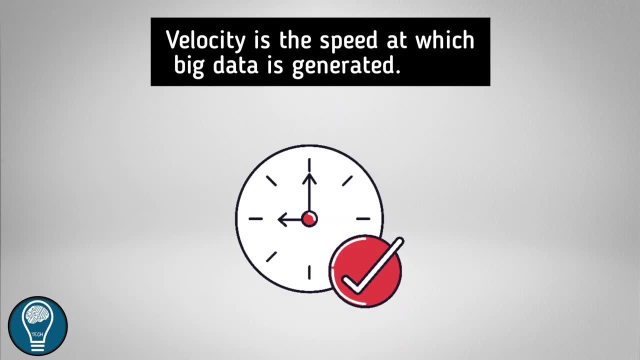 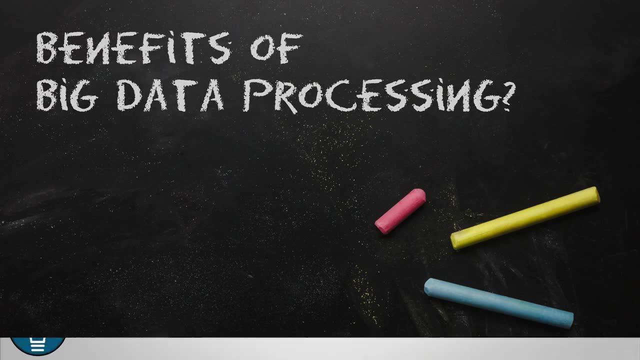 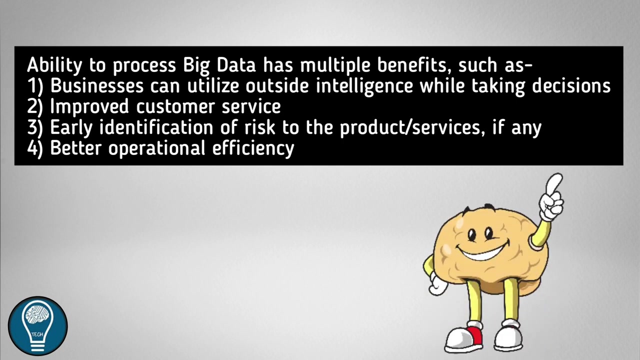 Variety contains types of data: Structured, semi-structured and unstructured. Velocity is the speed at which Big Data is generated. Let's get to the last part of the video, that is, benefits of Big Data processing. Ability to process Big Data has multiple benefits, such as: 1. Businesses can utilize outside intelligence while taking decisions. 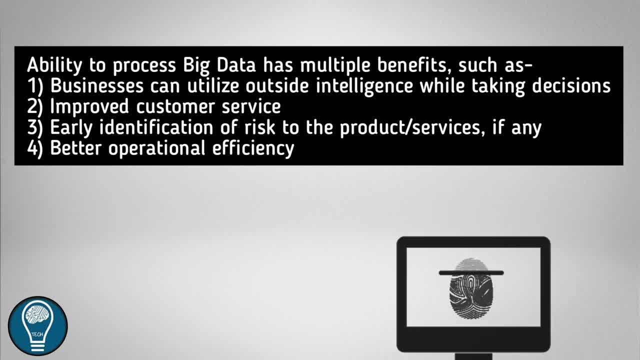 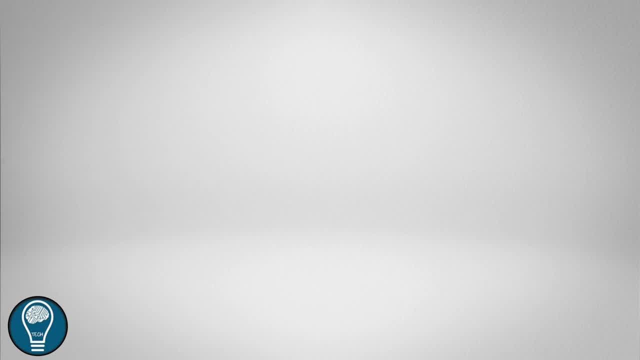 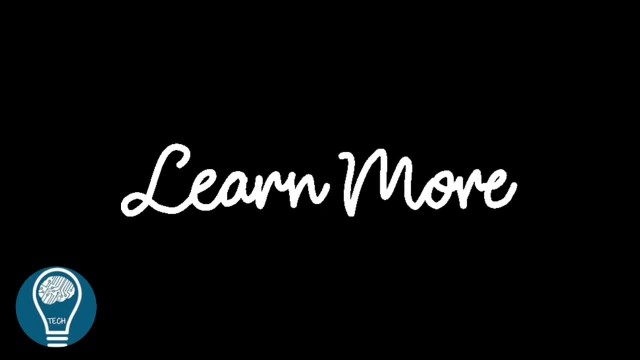 2. Improved customer service. 3. Early identification of risk to the product or services, if any. 4. Better operational efficiency. If you are new here, consider subscribing also to learn more. hit the bell icon to never miss an update from Meedy Technology.